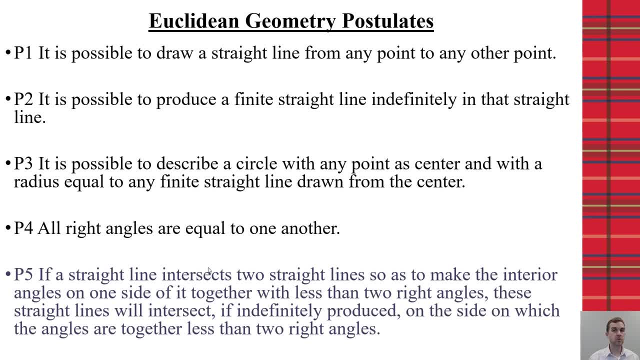 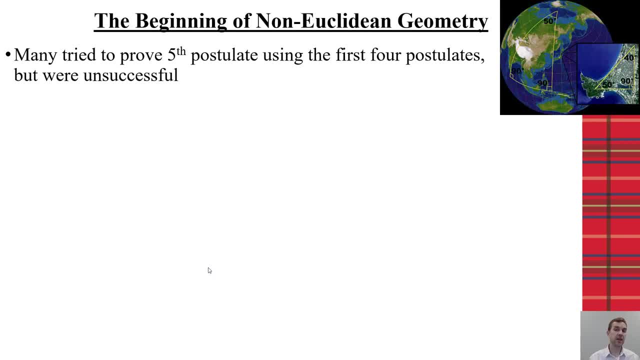 But the way that it was written by Euclid calls so many people to have concerns about. what does it really mean? And so many have tried to prove that fifth postulate using the other four postulates, but have been unsuccessful to do so. Hence why it is maintained over the millennium. 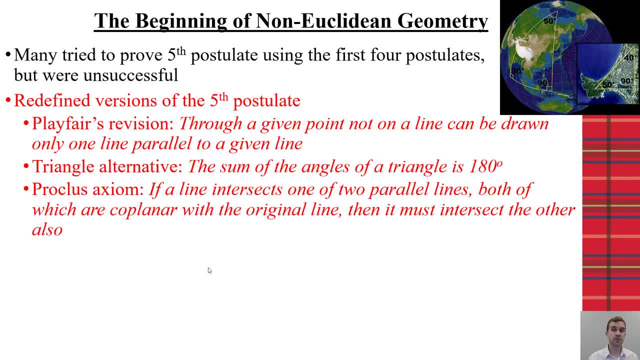 Now it has been revised many different times as people try to give us a better variation for what that postulate means. For example, Playfair said: Through a given point, not on a line, can be drawn only one parallel line to a given line, And that's true for Euclidean geometry, And that's often what we may even say within our own high school classes when we teach this. 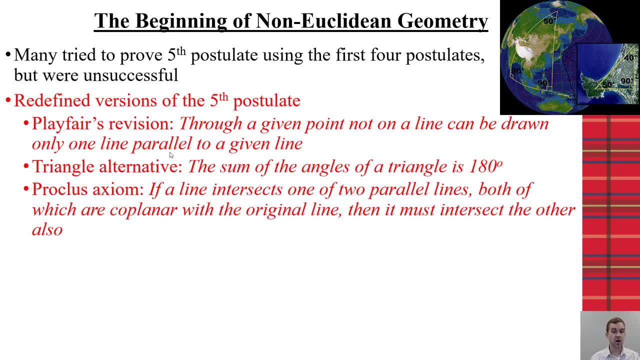 We have the idea that Proclus said: If a line intersects one of two parallel lines, both of which are coplanar to the original, then it must intersect the others also. So trying to look at it in a roundabout way, Now what this did by trying to look at all these different ways. 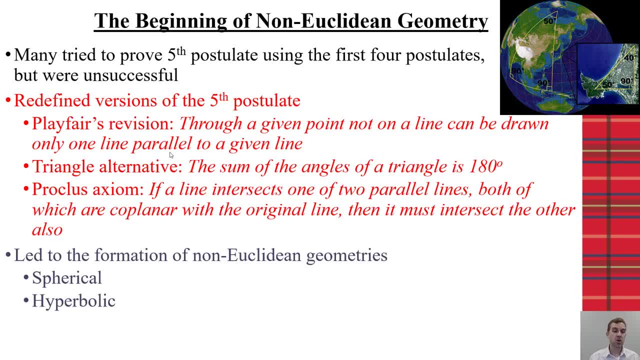 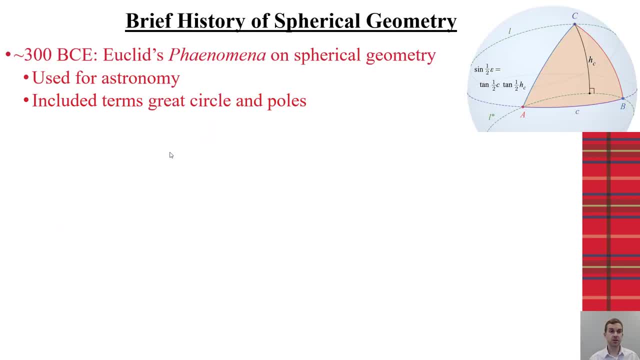 of understanding what this fifth postulate meant, created our non-Euclidean geometries that we consider especially spherical and hyperbolic geometry. The concept of spherical geometry has been around since the Greeks, Euclid actually wrote the phenomena, where he actually wrote about spherical geometry. 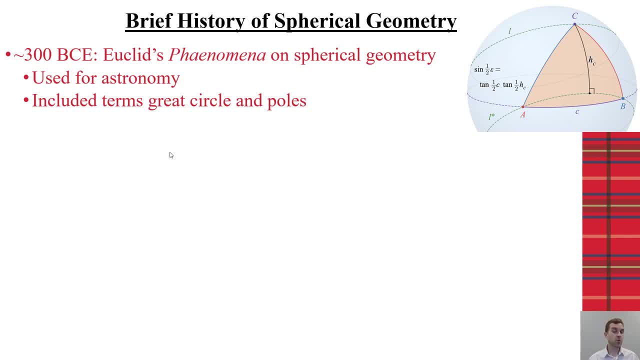 that was used for astronomy. It included terms like the great circle and poles and talked about the intersections of great circles and what would happen. Around 100 CE, Ptolemy constructed spherical maps that were on paper, so taking a three-dimensional concept and then transferring that to paper, and they were considered some of the greatest. 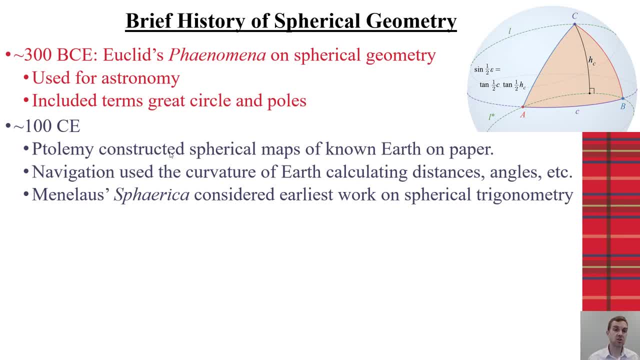 maps of that time. We know that they were using spherical geometry also for their navigation, as they were on their ships to help calculate their distances that they had to go, As well as Menelaus, around. that same time published the Spherical, which is considered. 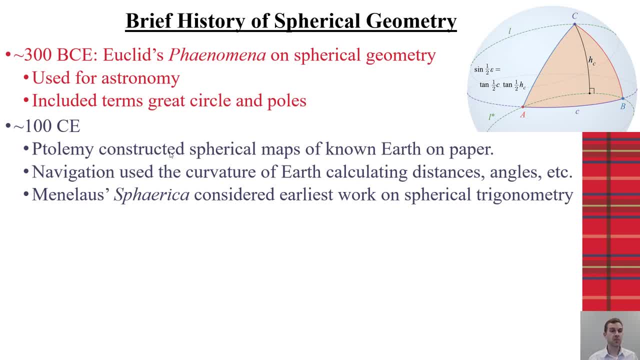 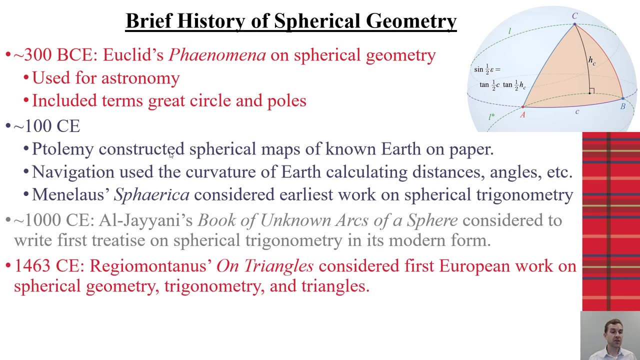 the earliest works of spherical trigonometry, Now around 1000 CE, We have the Muslim mathematician Al-Jayani, who published the Book of Unknown Arcs of a Sphere, And that's considered one of our first treatises of spherical trigonometry in its modern form. 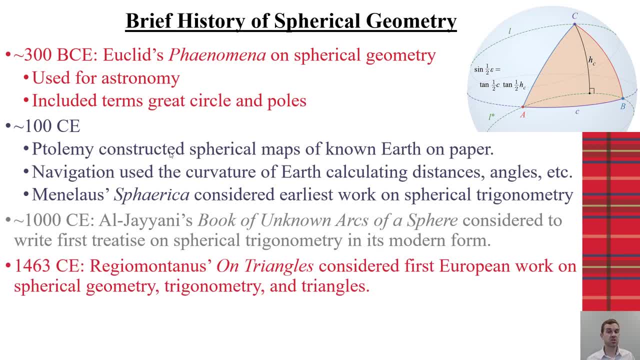 And then around 1463, Regiomontanus published On Triangles, which is considered the first European works on spherical geometry, spherical trigonometry and spherical triangles, And then the works that we often consider was spherical geometry now were put together. 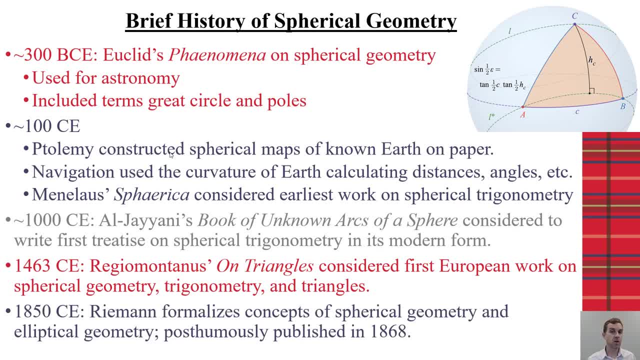 by Riemann in 1850. And then the works that we often consider was spherical geometry now were put together by Riemann in 1850. His work started as a lecture and then afterwards it was published after he died in 1868. 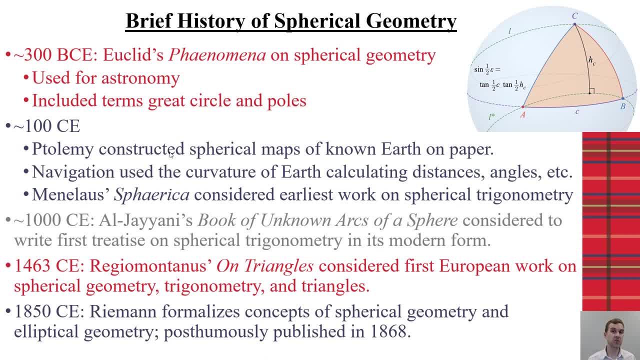 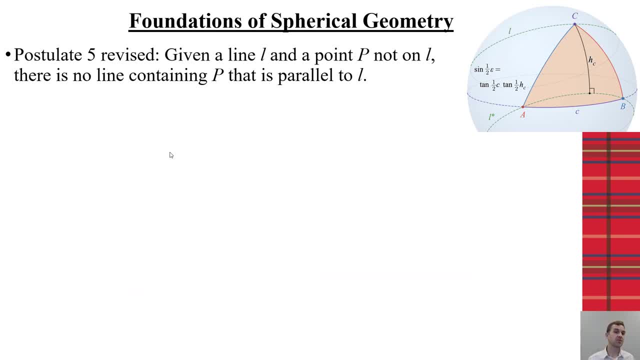 And those are the key works that we use now when we study spherical geometry. Now, when we think about what is spherical geometry, this revised postulate 5 to help us better understand what it means. So if we have a given line L and a point P that is not on L, there is no line containing. 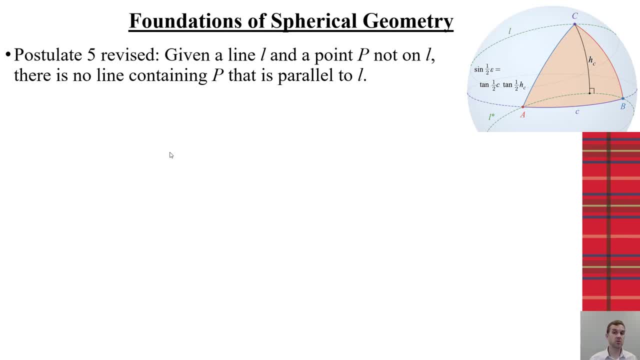 P that is parallel to L Because of the great circles. it gives us a key part that there are always intersections of our great circles. so there is no parallel lines. So a line is considered a great circle, so it has to be the circumference of the sphere. 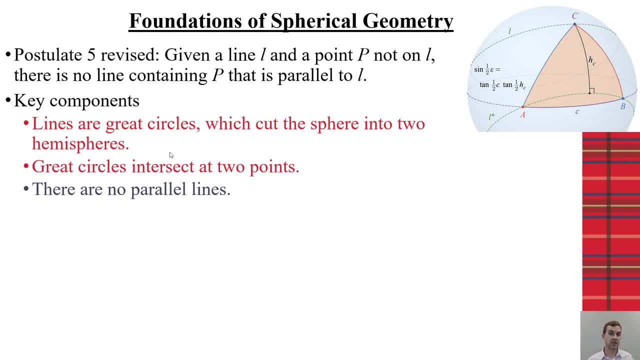 So they always intersect at two points, and it is impossible to create the circumference without creating another circumference that intersects. Now, by doing so, it changes how we think about our shapes. We think about them in Euclidean terms and those properties do not transfer the same. 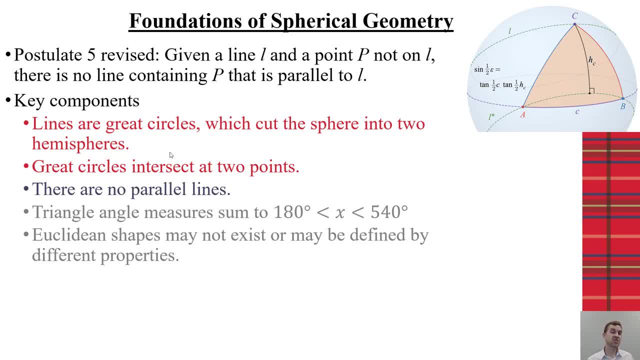 way. For example, triangle angle measures actually sum to somewhere between 180 and 540 degrees and they can change on how we make the triangle. Also, when we look at other shapes, they're not going to exist necessarily using the same properties that we see in Euclidean geometry. so you have to think about well what changes. 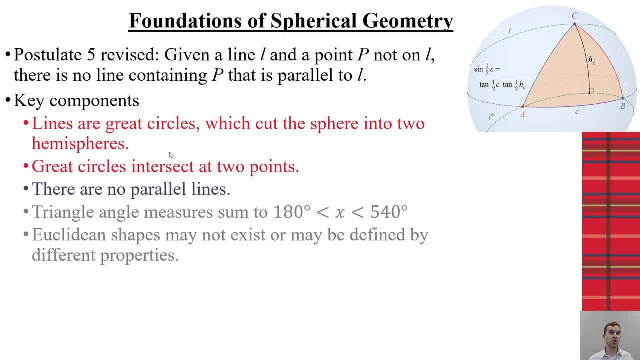 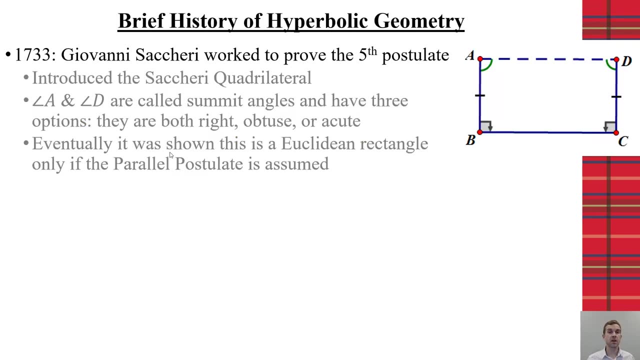 Do we still consider that to be, say, a rectangle if none of the sides are parallel, since we can't construct parallel lines in spherical geometry? or do we take the idea of a spherical rectangle and give it different properties that maybe can be utilized on the sphere? 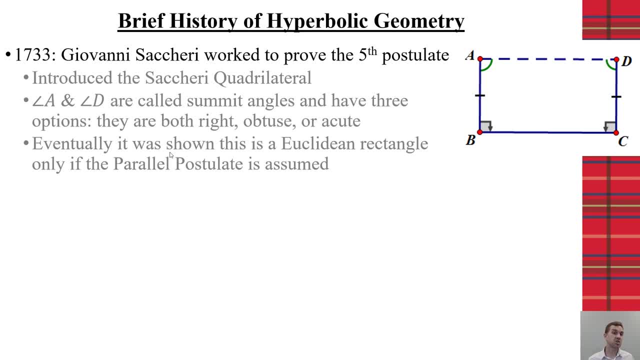 Now, when we look, then, at hyperbolic geometry, that had a much later start, say in 1733 CE, and even before that, people were playing with the idea of this fifth postulate and trying to figure out how do we get this idea of the acute angles? 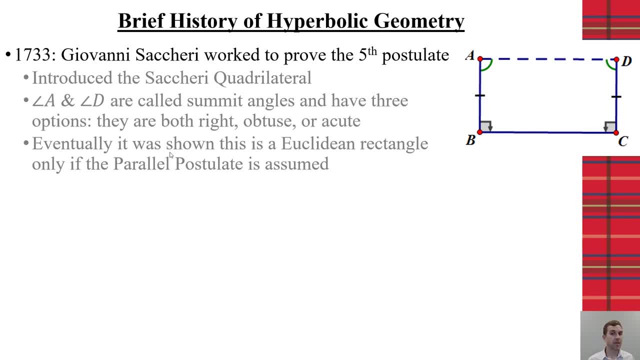 So Giovanni Sacceri, who was a professor at the University of Italy at the time. he worked around the idea of the fifth postulate and created the Sacceri quadrilateral, In that he fixed two angles as being right angles and then determined that the other 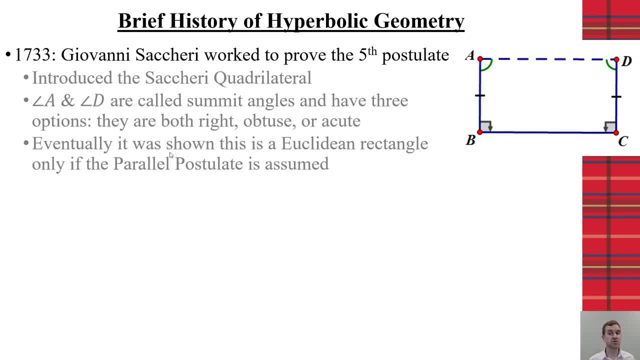 two, say A and D in this case, had to both be right, obtuse or acute. And with this that helps to show why the Euclidean triangle is only true if the parallel postulate is assumed. Now, with this work based on previous things that happened, Sacceri is able to go through. 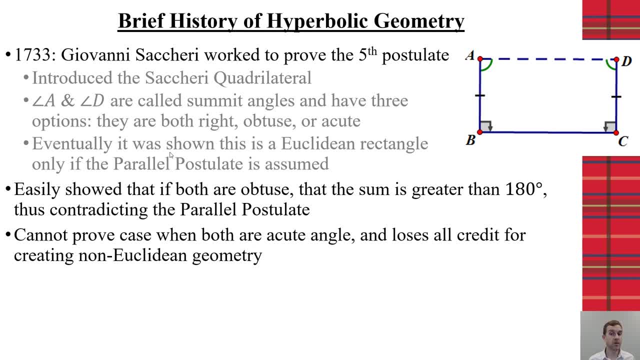 and show the obtuse category of why the sum is greater than 180 degrees, contradicting the parallel postulate, but can't get to the concept of having the two acute angles, And because he spent so much time trying to fight this ability to find the quadrilateral. 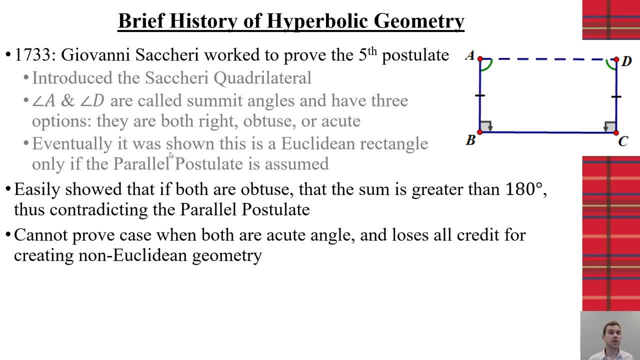 with the two acute angles, he lost his credit for what he'd been able to do in building the Sacceri quadrilateral. Now, after him, in 1777, Johann Lambert also continued to work on this And he took it to another step and said: there's three right angles, and let's look at that. 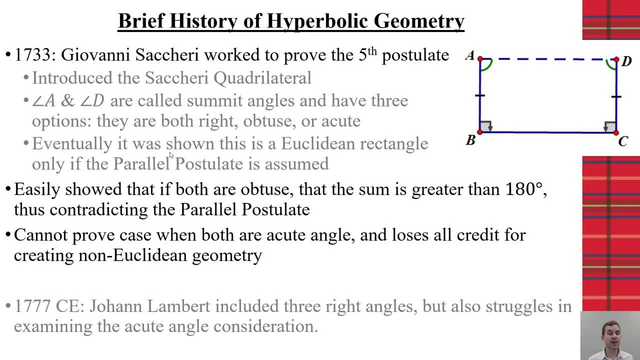 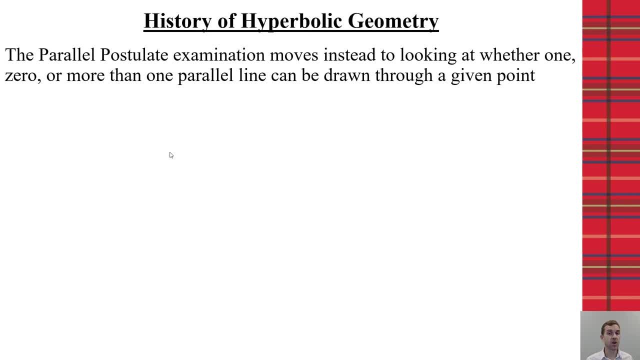 fourth angle, and what happens when we make it right, obtuse and acute. He too struggled with the idea of how to handle that acute angle in the consideration of this. Now, that then led to people examining whether there should be zero parallel lines, more than one parallel line, or exactly one. 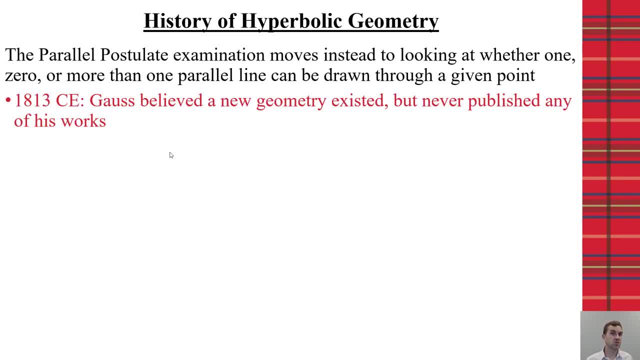 You get famous mathematicians such as Gauss, who started to examine The works of hyperbolic geometry. We know that Euler was working with spherical geometry in the 1700s, but Gauss is one that we often will hear. gave the term non-Euclidean geometry, coined that term, but he never actually 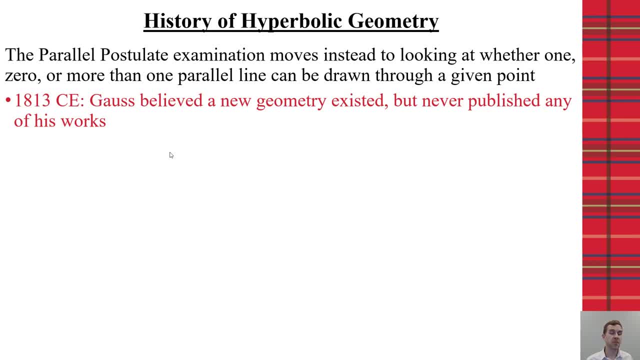 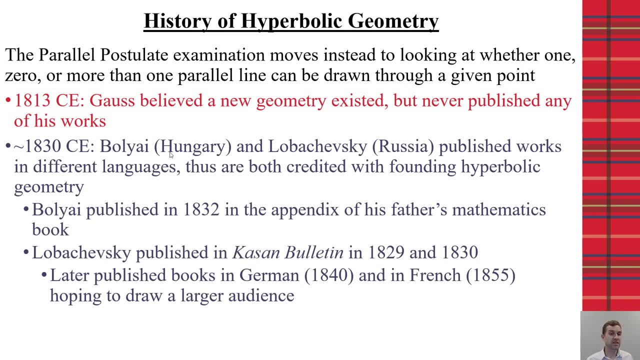 published anything related to what he thought about the geometry, So there's no credit that's given to him for his work. However, in 1830, around that time, we have two different mathematicians: Bolya and Hungry and Lobachevsky. 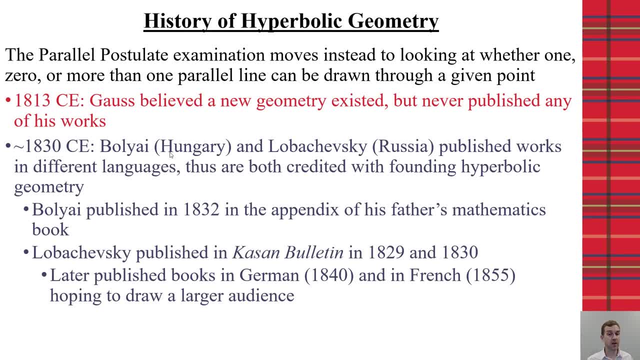 In Russia that published their work around the idea of hyperbolic geometry, and because they were in different countries, even though it's within a year or two and it wasn't actually overlapping, there's no way people can say that they stole their work from another person. 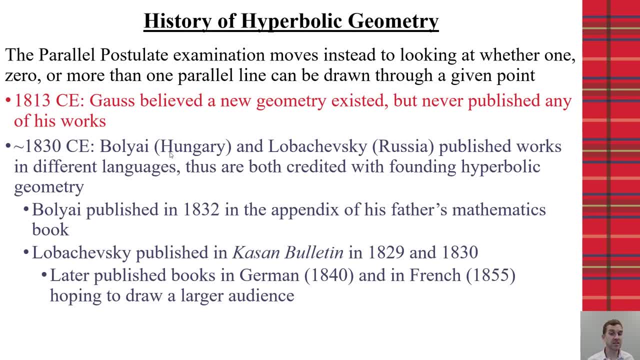 So that's why they're both credited with this work. Bolya published in 1832, Lobachevsky around 1829, 1830, and later published his works again in 1840 and 1855 to try to get more credit for the concepts of his hyperbolic. 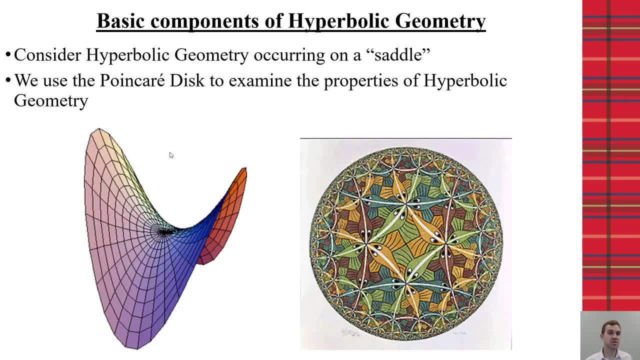 geometry And when we think about hyperbolic geometry, it's important to recognize what are we looking at, Because a spherical geometry makes a lot of sense to us. We have the sphere, We live on a sphere, which is why people created spherical geometry, most likely in the first 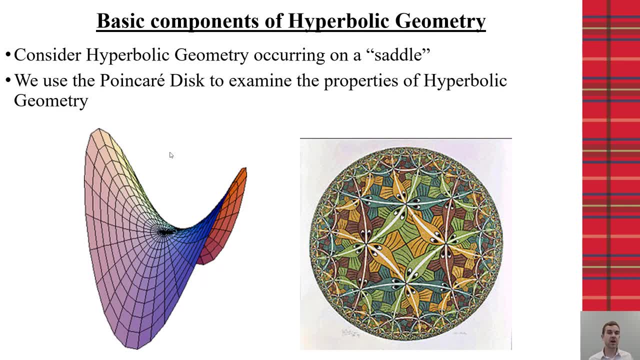 place The idea of the hyperbolic geometry. we look at it as if it was built on a saddle, And then, when we actually try to explore the properties of this, we use what's called a Poincare disk, And that allows us then to play with the different components. 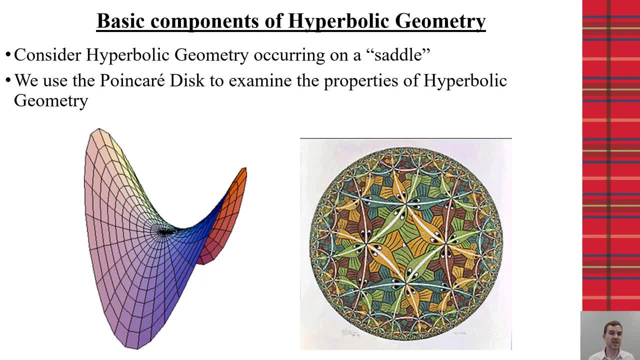 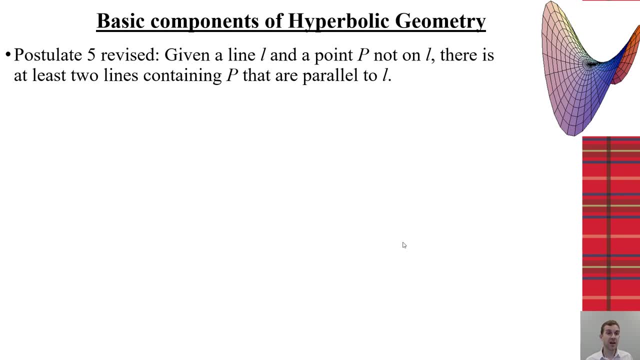 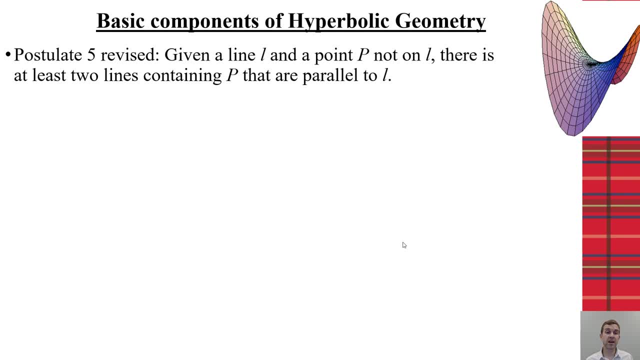 Now some of the key parts to understanding about hyperbolic geometry. It's revised. fifth postulate states that, given a line L and a point P, not on that line, there is at least two lines containing P that are parallel to L. What we're getting at here? 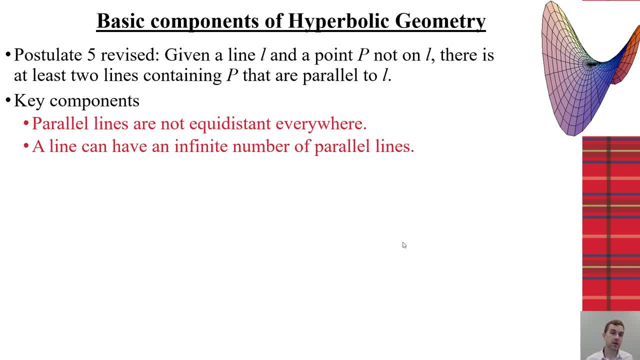 those. because of that, the way we consider parallel lines, they're not going to be equidistant everywhere, like we think about Euclidean parallel lines, where it's always an equidistant from one to the other, And it has to do with that fact that we're bending around the saddle Again. 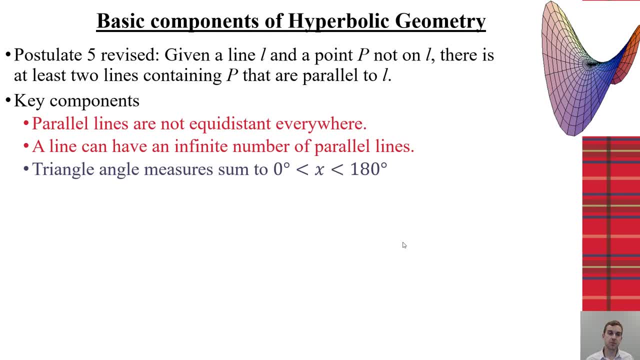 because of this curvature. the angles measures for a triangle are actually between zero degrees and 180 degrees and they can be changed depending on how we construct that triangle, which gives it unique properties. when we think about triangles And just like with spherical geometry, in the hyperbolic geometry, Euclidean shapes change yet again. So some properties we 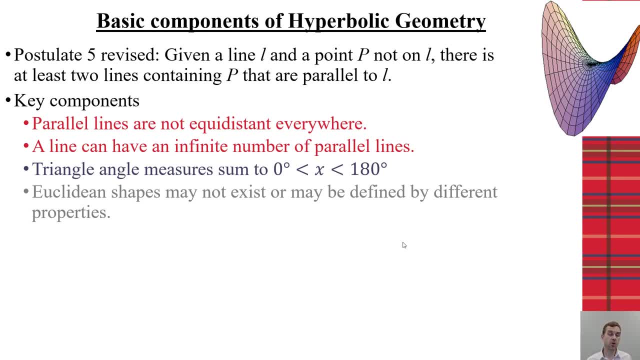 may consider may hold, but then other properties may not hold. We have to determine what is it we want to call this shape and do we still consider it by that same name?